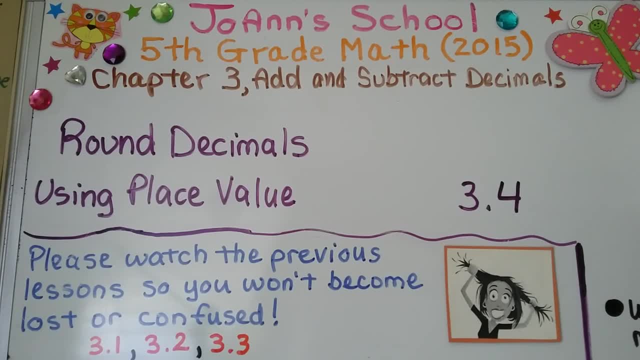 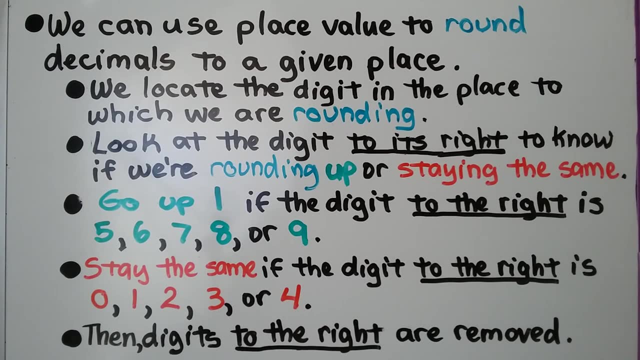 Lesson 3.4: round decimals using place value. We're also going to use a place value chart. We can use place value to round decimals to a given place. We locate the digit in the place to which we are rounding. We look at the digit to its right to know if we're rounding up or staying the same. 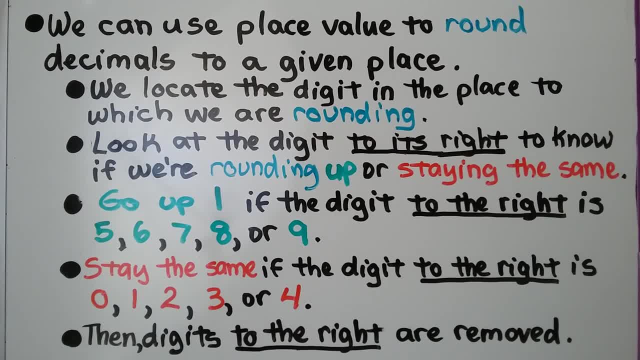 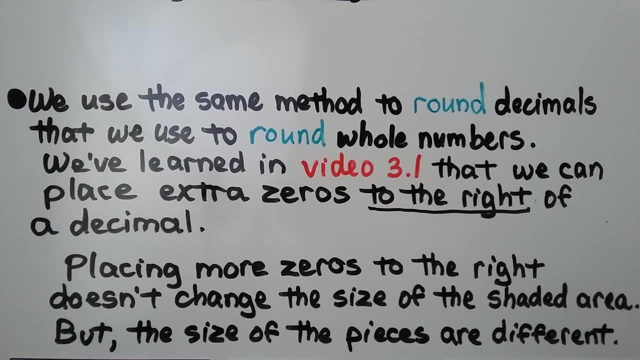 We go up one. if the digit to the right is a five, six, seven, eight or nine, We stay the same. if the digit to the right is a zero, one, two, three or four, Then digits to the right are removed. We use the same method to round decimals that we used around whole numbers. We've learned in 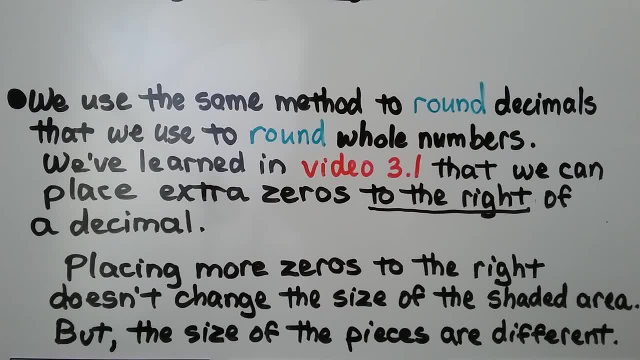 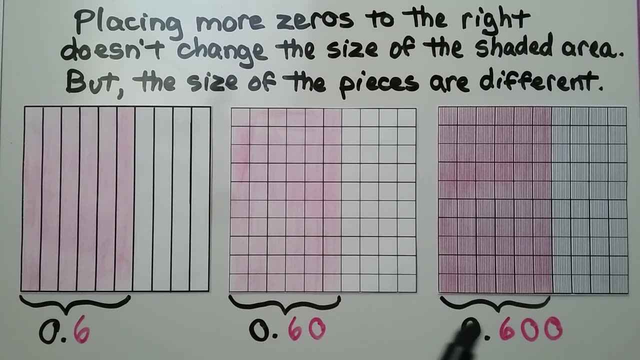 video 3.1 that we can place extra zeros to the right of a decimal. Placing more zeros to the right doesn't change the size of the shaded area, but the size of the pieces are different. For six tenths, sixty hundredths or six hundred thousandths, the same area is shaded, The size. 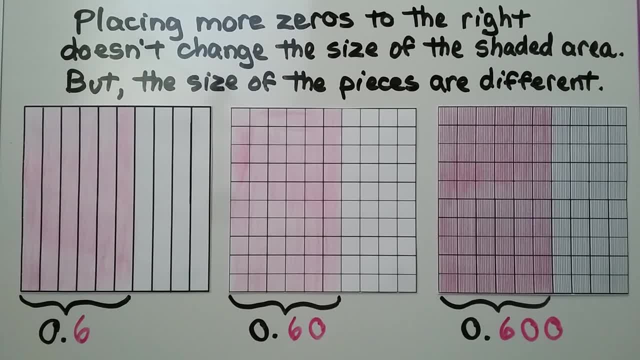 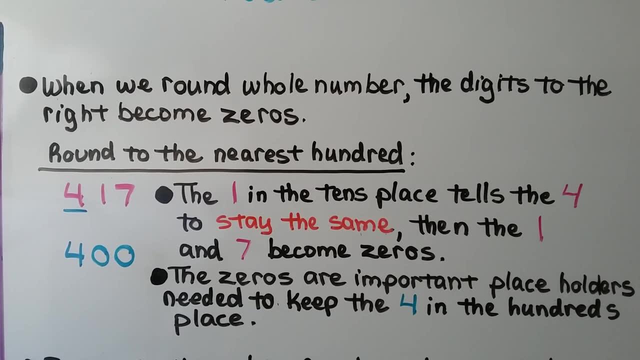 of the pieces are different, that's all. They each have a six in the tenths place. All of these decimals represent the same amount. When we round whole numbers, the digits to the right become zeros. We want to round to the nearest number. The decimal has to be more than the number. The 1 in the tenths place tells the four to. 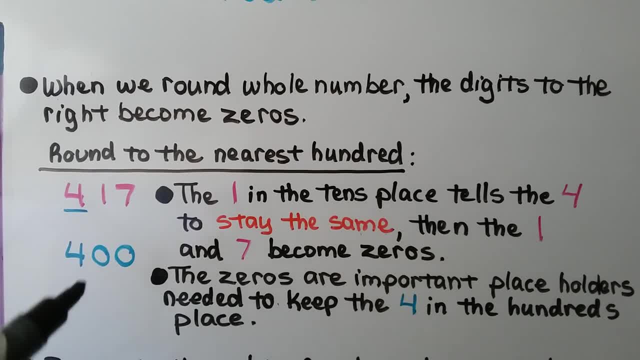 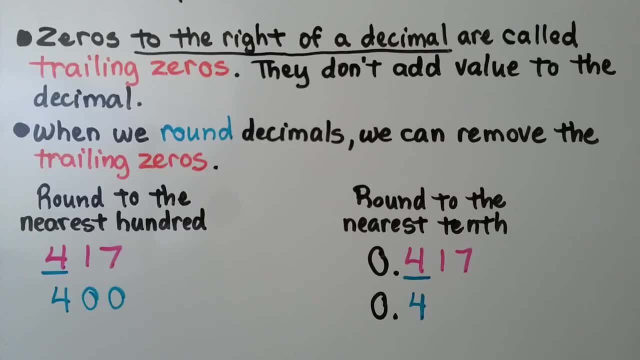 stay the same. The 1 and the 7 are zeros. The zeros are important placeholders to keep the four in the hundredths place. Zeros to the right of a decimal are called trailing zeros. They don't add value to the decimal. When we round decimals we can remove the trailing zeros. 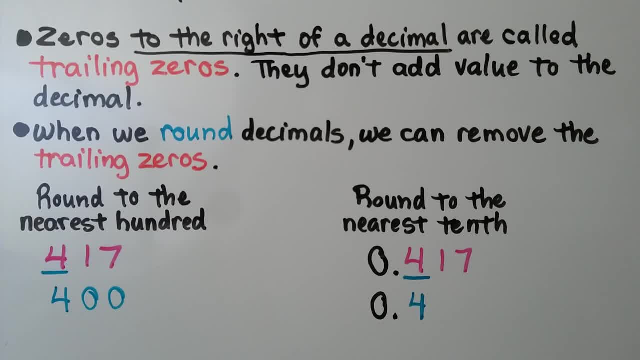 When we round decimals we can remove the trailing zeros. The 1 and the sevens are important to keep the fours in the hundredths place. So when we were rounding to the nearest hundred for the whole number, we needed the zeros to keep the four in the hundredths place. 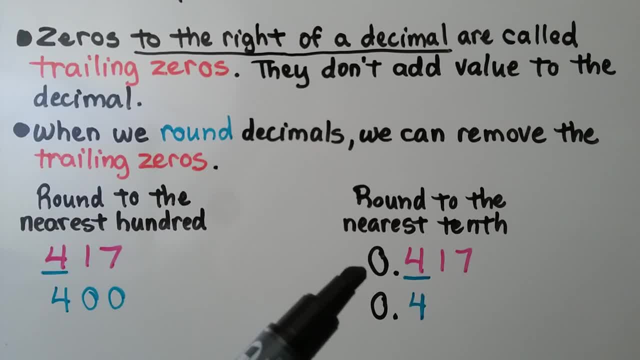 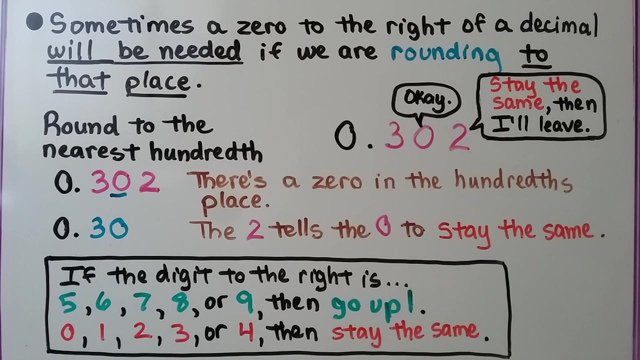 If we are rounding four hundred seventeen thousandths to the nearest tenth place, we can drop off the trailing zeros and write four tenths. The one in the hundredths place told the four to stay the same and they became zeros or nothing, and we can drop off those trailing zeros and just write four tenths. 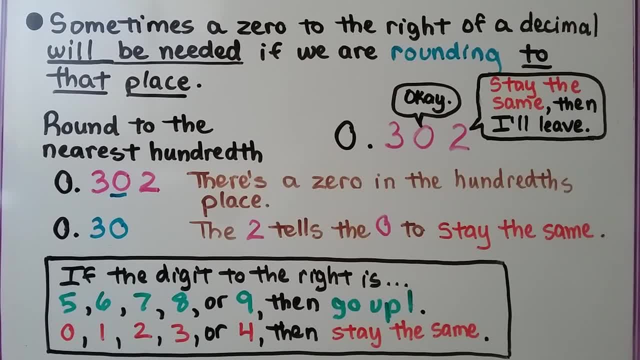 Sometimes a zero to the right of a decimal will be needed if we are rounding to that place. We're going to be rounding three hundred two thousandths to the nearest hundredth place. The two tells the zero to stay the same and then he is removed. 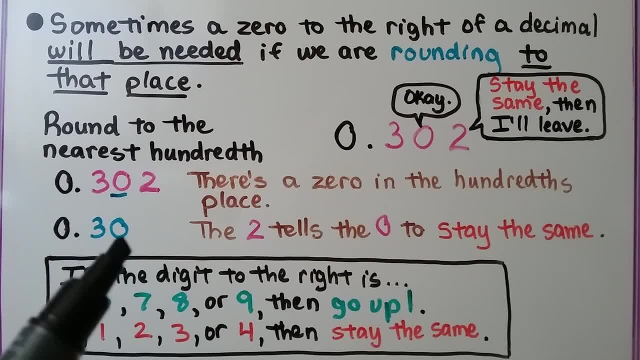 There's a zero in the hundredths place. The two tells the zero to stay the same and is removed. It rounds to thirty hundredths because we were rounding to the hundredths place. We need that zero to hold the hundredths place as a placeholder. 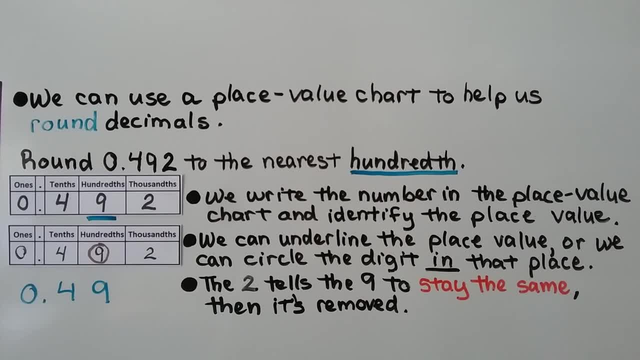 We can use a place value chart to help us round decimals. We need to round four hundred ninety-two thousandths to the nearest hundredth. We write the number in the place value chart And identify the place value We're rounding to the hundredths place. so we're rounding this nine to the hundredths. 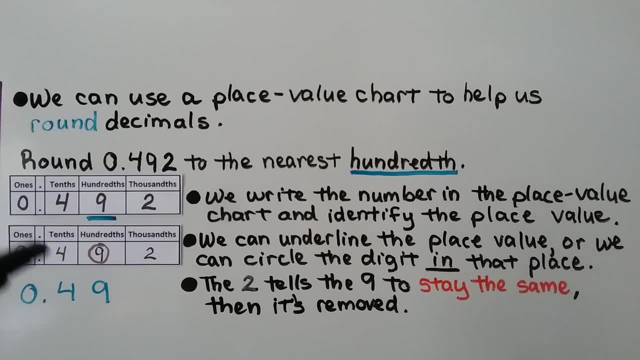 place And we can underline the place value or we could circle the digit in that place to help us identify it. The two tells the nine to stay the same. then it's removed. It rounds to forty-nine hundredths If we need to go up one. . . . . . . . . . . . . . . . . . . . . . . . . . . . . . . . . . . . . . . . . . . . . . . . . . . . . . 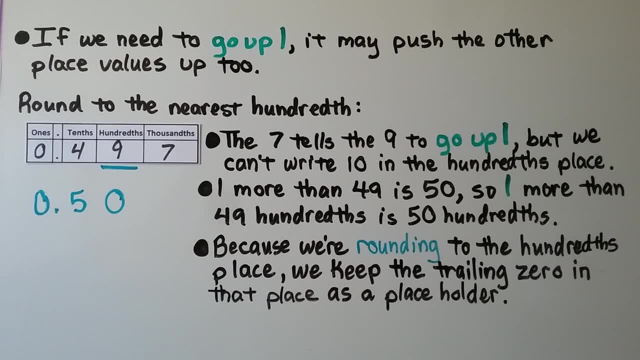 Another place value is up two. Round to the nearest hundredth we have four hundred ninety-seven hundredths. The seven tells the nine to go up one, But we can't write 10 in the hundredth place…. 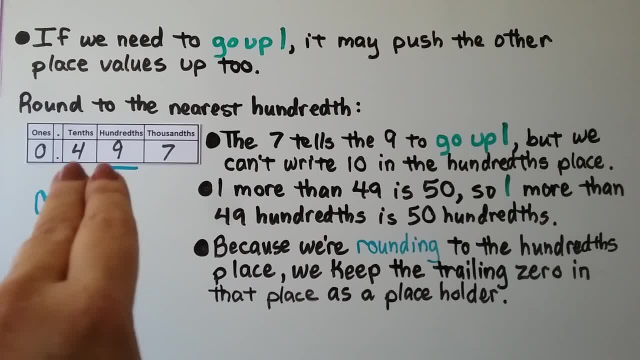 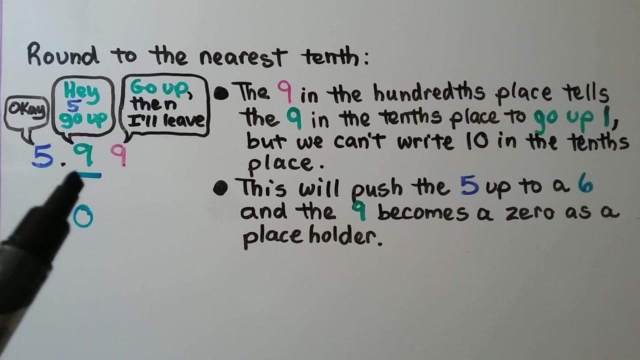 And one more than 49 is 50, so one more than 49 hundredths is 50 hundredths And because we're rounding to the hundredth place, we keep the trailing zero in that place as a placeholder. We need to round to the nearest tenth. We have 5 and 99 hundredths, The 9 in the hundredths place. 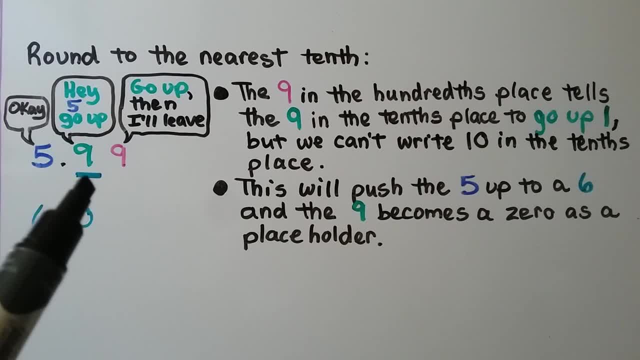 tells the 9 in the tenths place to go up one. but we can't write 10 in the tenths place. This will push the 5 up to a 6 and this 9 will become a 0 as a placeholder and this 9 drops off. So the 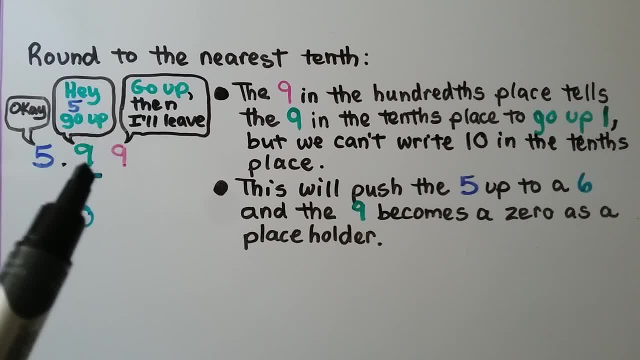 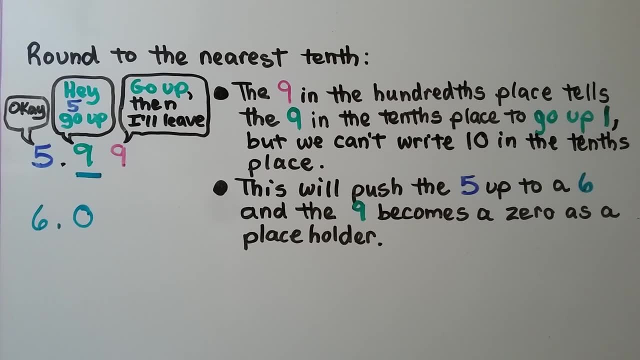 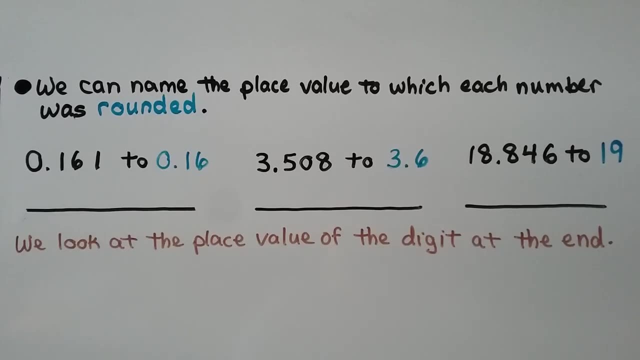 9 said: go up and then I'll leave. and he said: hey, 5 go up. and the 5 said: okay, It rounds to 6 ones as 6 and 0 tenths We can name the place values to which each number was rounded. We have 161 thousandths and it was rounded to 16 hundredths. 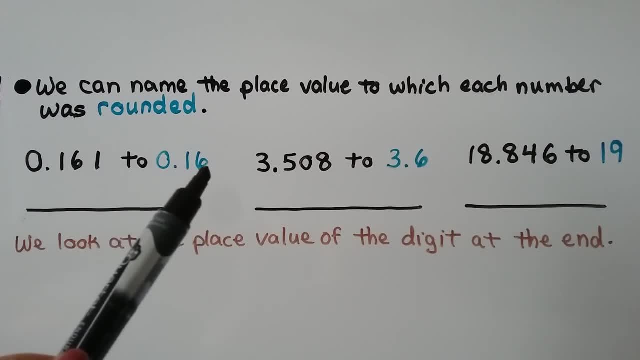 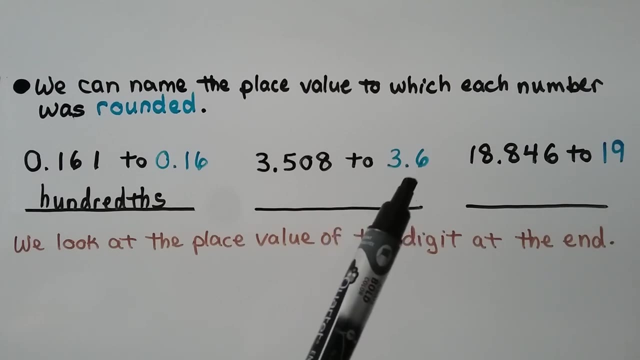 We look at the place value of the digit at the end, It's in the hundredths place. This was rounded to the hundredths Here. 3 and 508 thousandths was rounded to 3 and 6 tenths. We look at the place value of the digit at the end. It's in the tenths place. 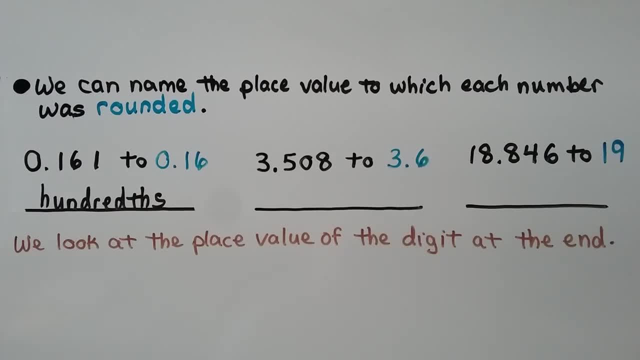 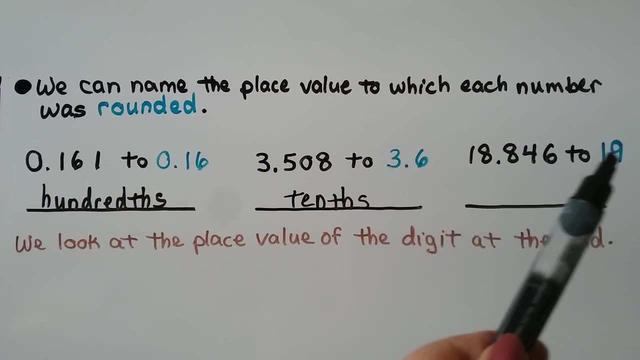 We know this was rounded to the hundredths. Here we have 18 and 846 thousandths and it was rounded to 19.. We don't see any decimals. It was rounded to a whole number, 19.. We look at the place value of the digit at the end. It's a 9 in the ones. 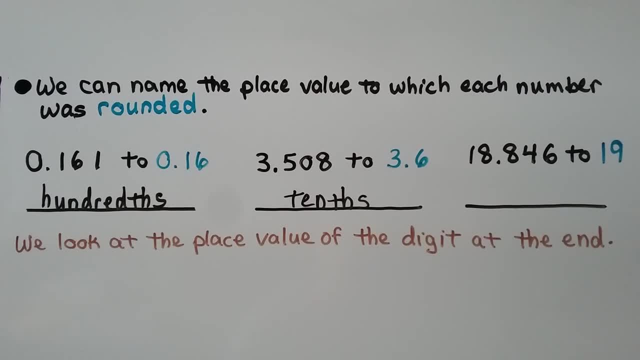 place It was rounded to the ones place. So all we had to do is look at the place value of the digit at the end and we knew which place value each number was going to be. So we knew which place value each number was rounded to. 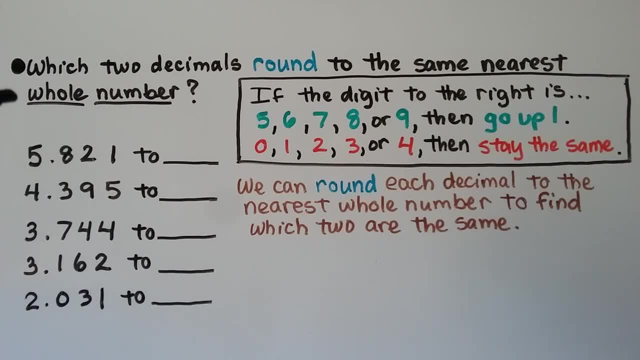 Here we have a lot of decimal numbers and it says which two decimals round to the same nearest whole number. So the whole numbers are to the left of the decimal point. We can round each decimal to the nearest whole number to find which two are the same. 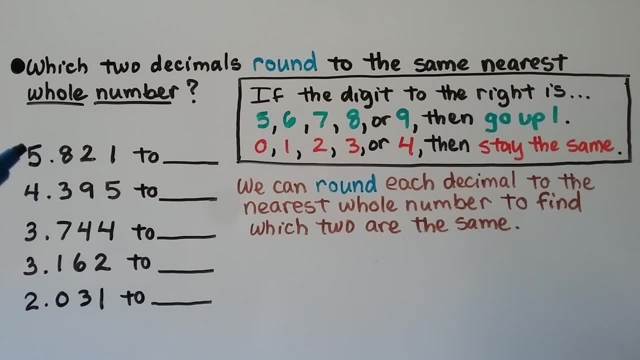 For this one we look to the right and the 8 is going to tell the 5 to round up one more, So it's going to round to six ones Here. the 3 in the tenths place is going to tell the four ones to stay the same. 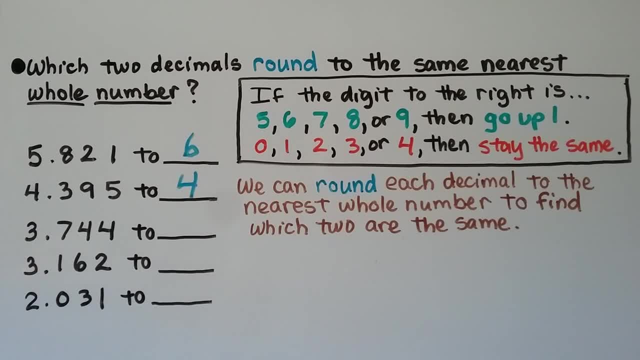 So it's going to round to four ones Here. the 7 in the tenths place is going to tell the 3 in the ones place to round up one. So it's going to round to four ones Here. the 1 in the tenths place tells the 3 in the ones place to stay. 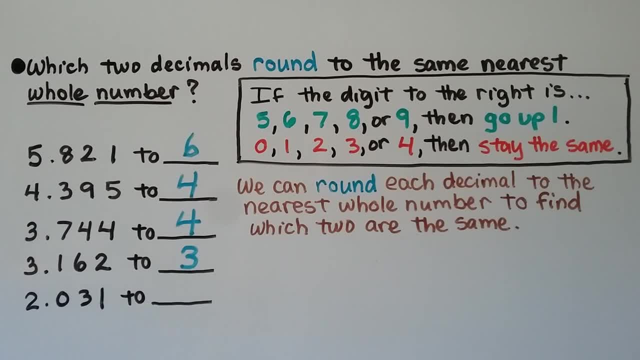 the same, So it rounds to three. Here the 0 in the tenths place tells the 2 to stay the same, so it rounds to two. And we can see which two decimals round to the same nearest whole number: 4 and 395 thousandths and 3 and 744 thousandths. both round to the whole number four. 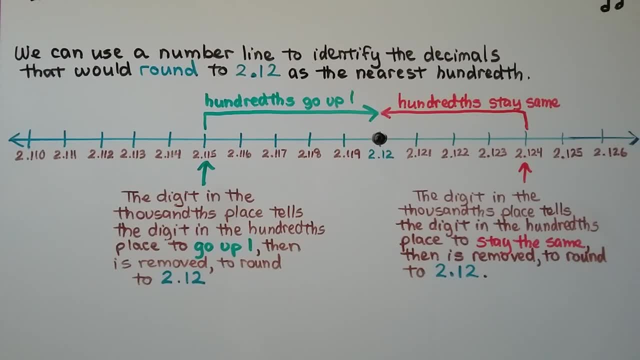 We can use a number line to identify the decimals. that would round to two and twelve hundredths as the nearest hundredth We can see they're written in thousandths. Here is two and twelve hundredths. Its trailing. zero was removed And the digit in the thousandths place tells the digit in the hundredths place. 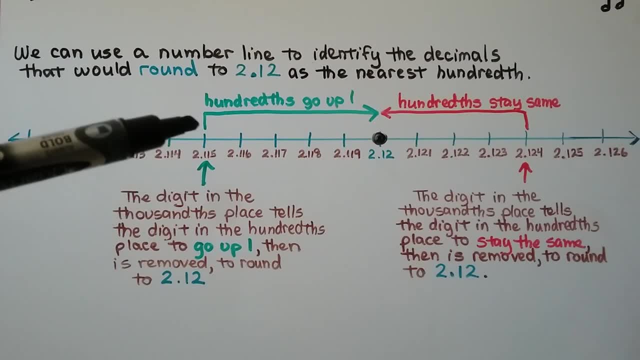 to go up one and then is removed and it rounds up to two and twelve hundredths From here, because we have a four. the digit in the thousandths place tells the digit in the hundredths place to stay the same, then is removed to round to two and twelve hundredths. 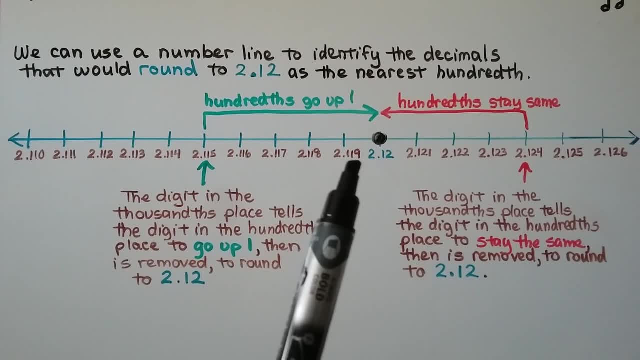 So these digits with a five, six, seven, eight, nine in the thousandths place will round up to two and twelve hundredths. And these digits with a one, two, three or four in the thousandths place tell the hundredths to stay the same as two and twelve hundredths. 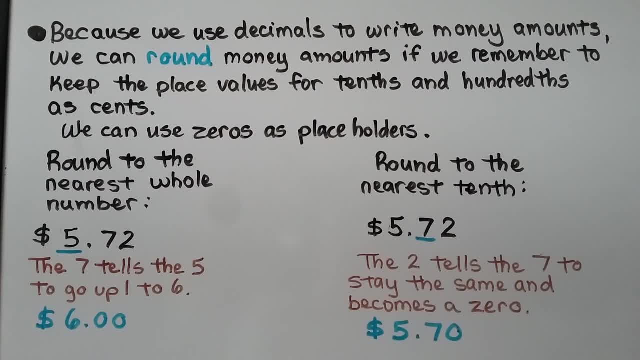 Because we use decimals to write money amounts. we can round money amounts if we remember to keep the place values for tenths and hundredths as cents. We can use zeros as placeholders. We need to round to the nearest whole number. This seven tells the five to go up to a six.